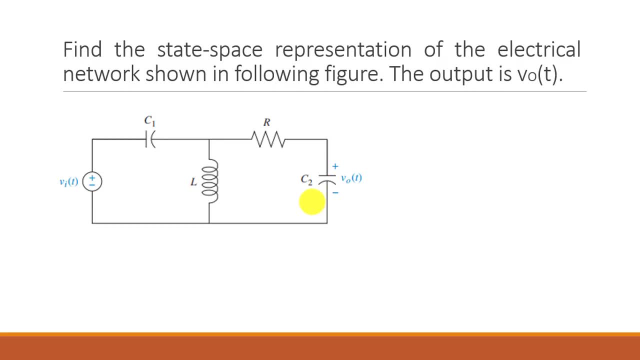 the very first thing that you have to identify is the state space variables. So state space variables matrix is the very first thing that we need to build. So identifying the components over here which can be represented in form of derivatives and equations are: 3. C1: this capacitor. 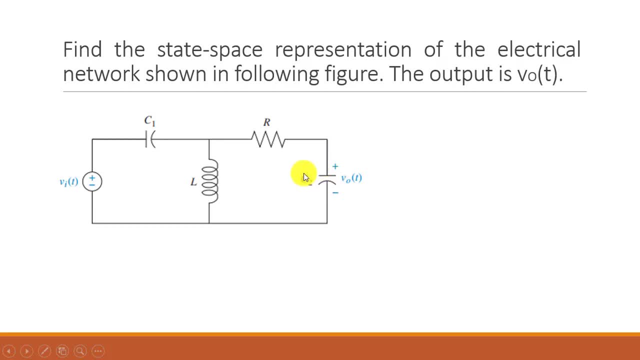 this inductor, L and C2, this capacitor. So we have two capacitors and one inductor. So we have three energy storage elements over here. Two of them are capacitors And one of them is inductor. Now we clearly know that capacitors resist change across their 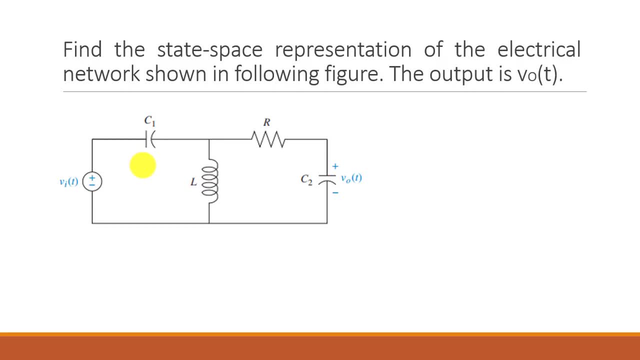 voltages and inductors resist in change in current across their endpoints. So we will have VC1, IL and VC2 as the major components of our state space matrix. So that's in front of you. The X matrix, the state space variables matrix, is VC1, IL, VC2.. And we know that X dot would be VC1 dot, IL, dot. 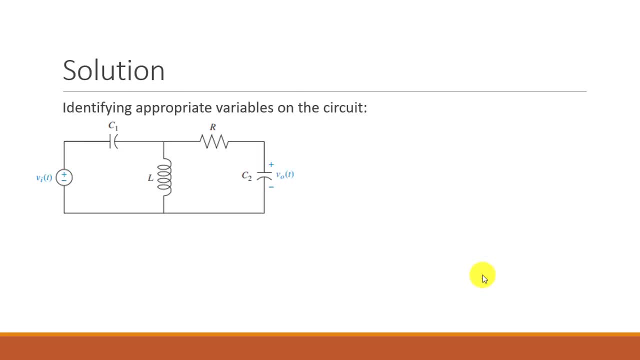 and VC2 dot. Now we move further toward writing the equation. The very first thing that we'll be doing after identifying the X matrix is that we have to identify the appropriate variables on the circuit. So you can see that I have mentioned the IC1, the inductor current, the capacitor 2 current and the resistor current over. 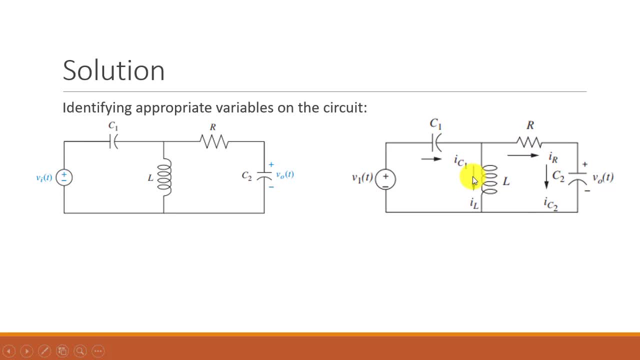 here And now we need to write equations for the state space variables that we had already mentioned in the very first slide. So the derivative relations for the capacitor is, we know, DVC divided by DT, that is, the change in voltage across a capacitor is basically equal to Ic1, that is, the current across it divided. 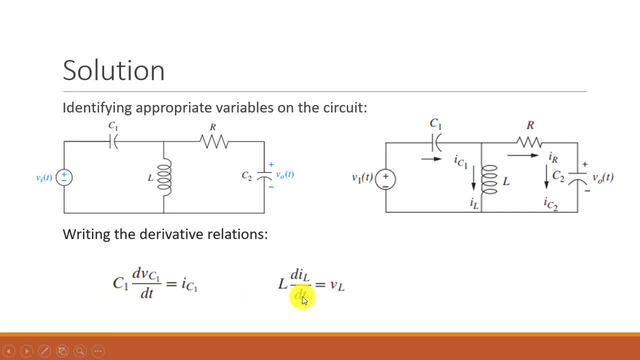 by the capacitance. Similarly, if we have an inductor, the change in its current is basically represented as the voltage divided by its inductance. and because we have two capacitors, one of them is named as C1 and the other one is named as C2, so we have written the equations for 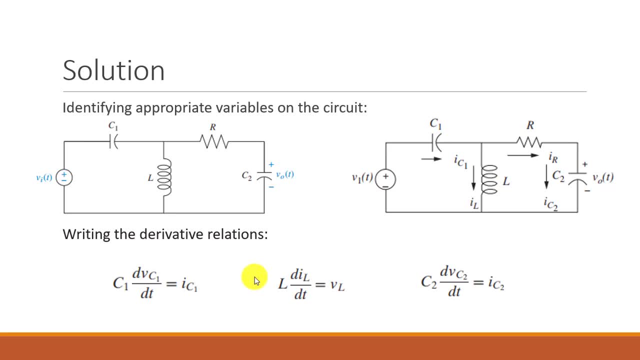 all of the components, all of the state variables that we have. Now we need to find out these terms- Ic1, VL and Ic2- with respect to this diagram that has been given to us. So, if you can see closely, in this diagram I have already depicted Ic1, IL, IR and Ic2 and, with the help of Kirchhoff's, 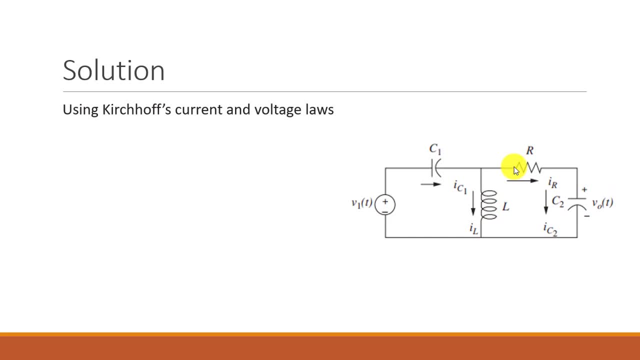 current law and voltage law. we'll write the equations that are given to us. So the Ic1 current is basically- if you see closely in this figure, is sum of IR plus IL. The capacitor 1 current is basically the sum of current that's flowing through this resistor. 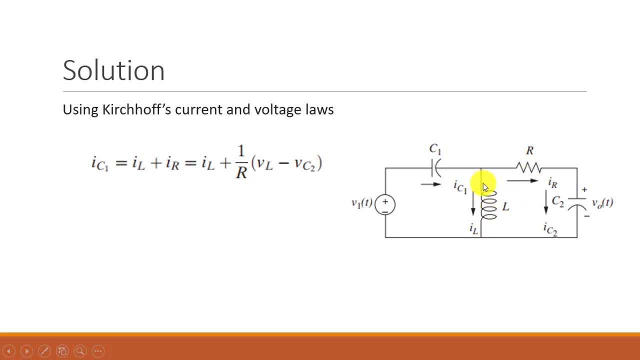 and this inductor. Now we can see that the resistor current, this IR, is basically nothing but a value which is flowing due to the difference of voltages that are being developed across this inductor and this capacitor. So the voltage across this inductor is VL and across this capacitor is 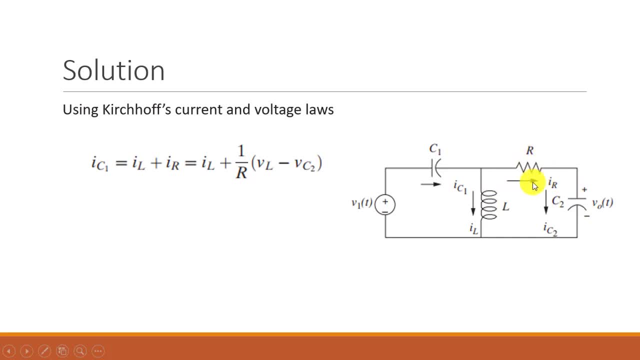 VC. So VL minus VC divided by this impedance, that is, the R, is basically equal to the current that's flowing through this resistor, IR resistor R. So we put in the values of IL as it is and IR as 1 R into VL minus VC2.. Considering that the voltage in this inductor is greater than the voltage across, 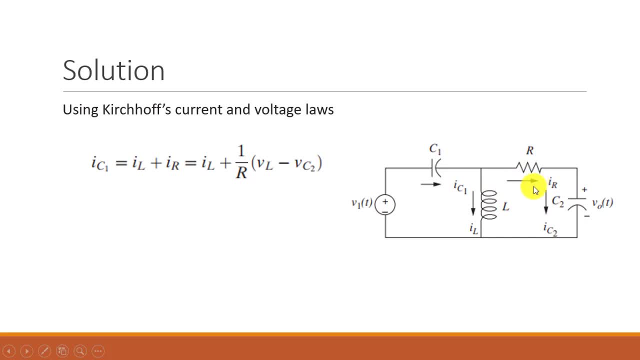 this capacitor because the current is flowing towards the rightward direction, as we have chosen initially. If we choose different directions, the signs would change and at the end, all of that would equally be right. You can change the directions, there would be different signs, but the result 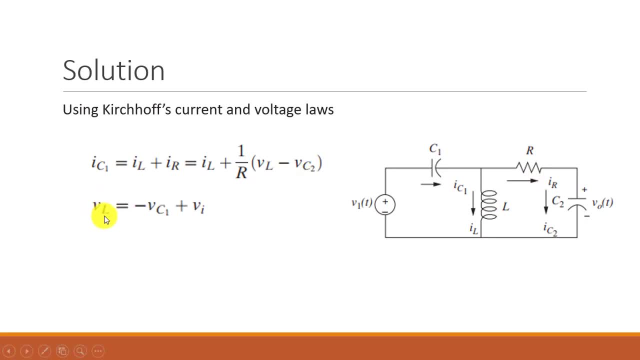 would be same. So the next thing is VL, because I told you that we have to find out equations for the terms that had been mentioned in the derivative relations. So we know that change in current is in derivative form for the inductor. So we need to find out the voltage relation and we can see that VL, the voltage that is being developed. 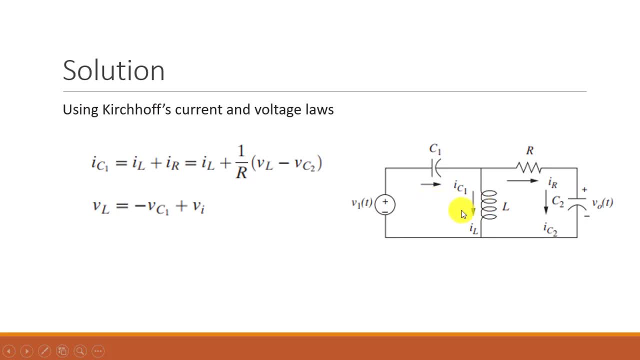 at this inductor is nothing but the sum of this voltage minus the capacitor drop. So this voltage minus the voltage which is being dropped at this capacitor would be equal to the voltage at this inductor because they are in parallel. So VL is equal to minus VC1 plus VI. Next thing is the. 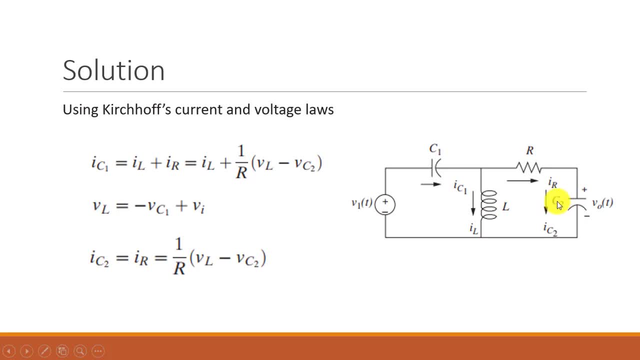 capacitor, current IC2, and if you see that, because this capacitor is in series with this resistance R. So IC2 is basically equal to IR, and we already know from the very first equation that IR is nothing but 1 over R into VL minus VC2.. So this is the third equation. then the only thing that's left now is that we have 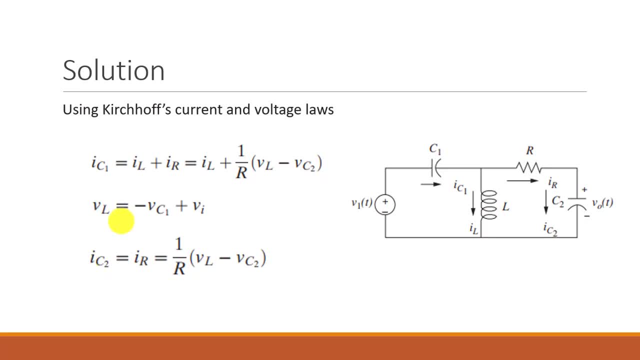 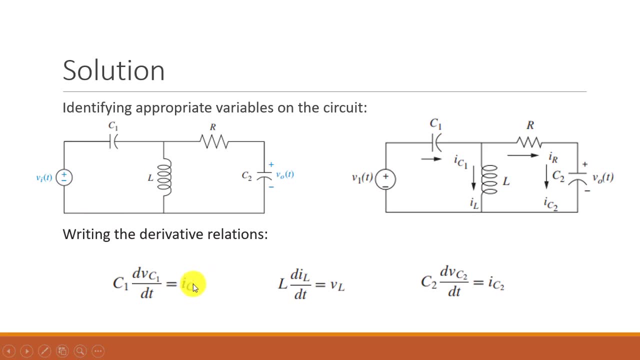 to put these three equations, these three relations, where, here in these, in these three equations, relations that we have mentioned, we have found out IC1, we have find out, found out VL, we have found out IC2.. So we just put in the values over here in this relations that we are, that we have. 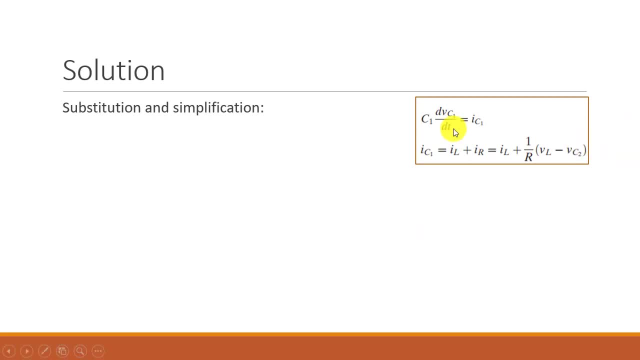 been given already. So the very first relation that we are looking at is the current voltage IC1 relation and this equation that we found out in the previous section. So you can see that if we put in the value of IC1 in this equation, C1 would be divided by all the terms that are on the right. 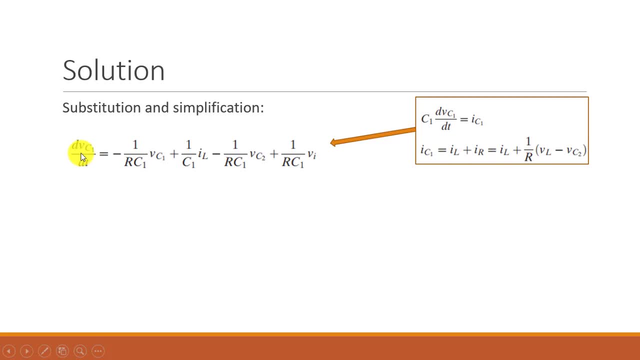 side and DVC1 divided by DT would be on the left side. This is nothing but VC1 dot and that would be the derivative component of the VC part that's already in RX matrix, the state space matrix. the next relation that we are going to use are 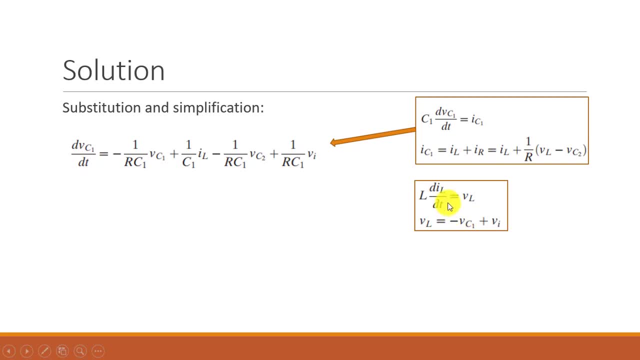 the voltage of inductor ones. so we put in the value of VL into this equation and the result is in front of you. we have put in the value of VL over here from here, minus VC1, plus VI, and both of them are divided by inductor impedance. 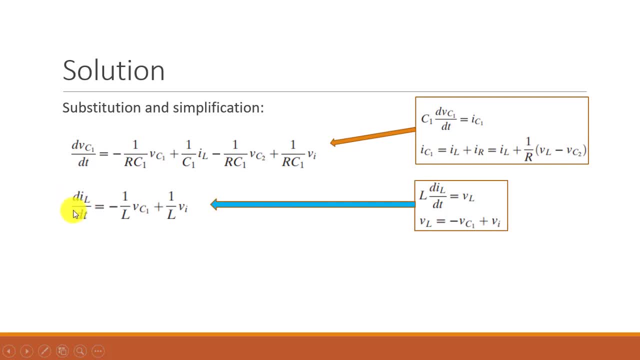 L, inductance L, and here would be IL, dot, or you can say the derivative of current that's being flowed through the inductor. the next relationship set of relationship is for the IC2 and will follow the same trend that we have been following in the previous two relations, so we'll just put in the values over. 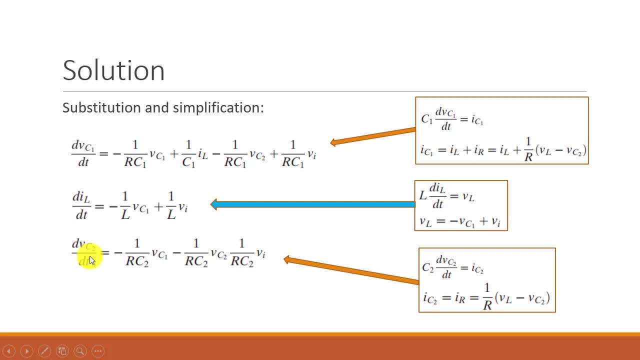 here and we have the equation for VC2 dot. now you can see that the three state space variables that we had divided by the current value of VL over here are developed in the very first look at the question. now we'll just put in the values in the matrices to find out the matrix A, matrix B, matrix C and matrix D. 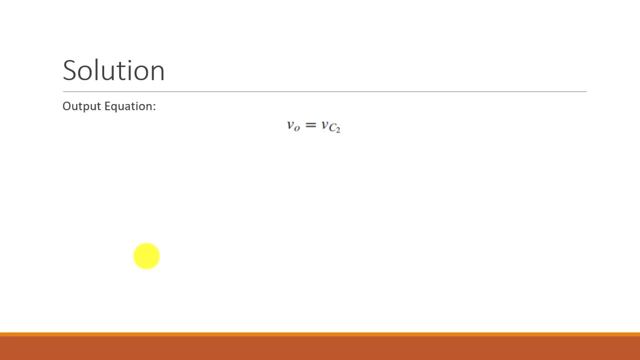 you can in the equation, you can in the question we have. we know that it was given that output is V out, which is the voltage that was being developed at the capacitor C2. so V out is basically nothing but VC2. now we put in the values into the X dot is equal to AX plus BU. so this is the A matrix and 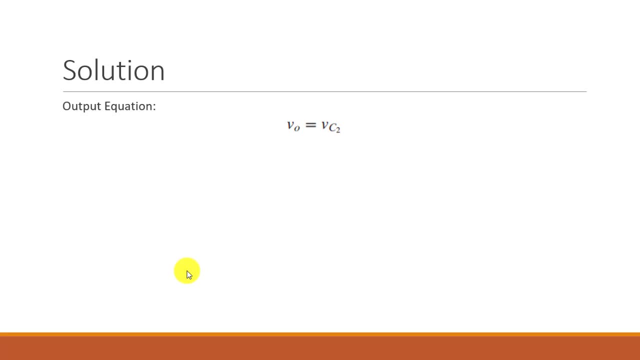 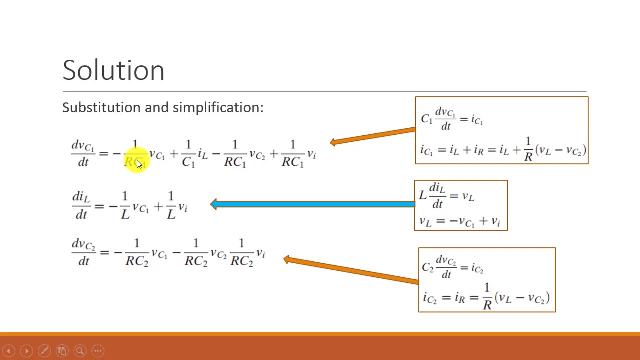 how have we filled it? we have filled this matrix using these equations, these three equations for VC 1 dot. you can see- I will just show to one of the values- VC 1 dot is equal to minus 1 over RC1 into VC 1. and if we have a look at the X, 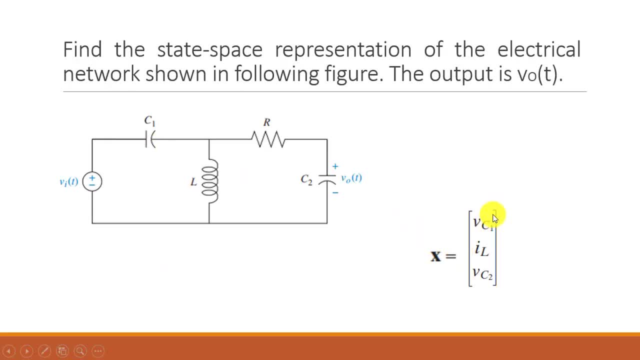 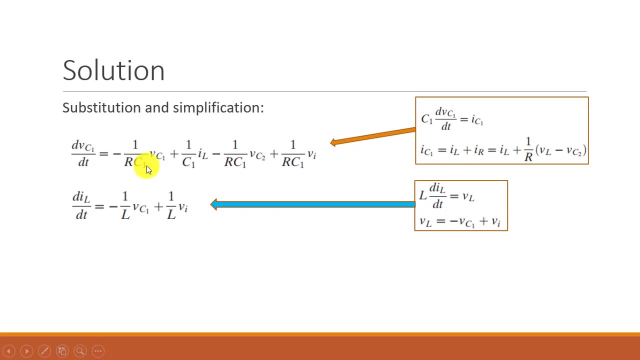 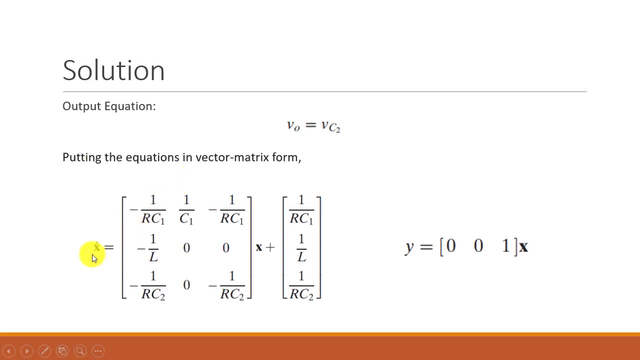 metrics. you can see the X method has the very first component as VC1. So VC1 has the coefficient minus 1 over RC1 in the VC1 dot equation, which is the very first equation, and you can see that the VC1 dot equation that would be: 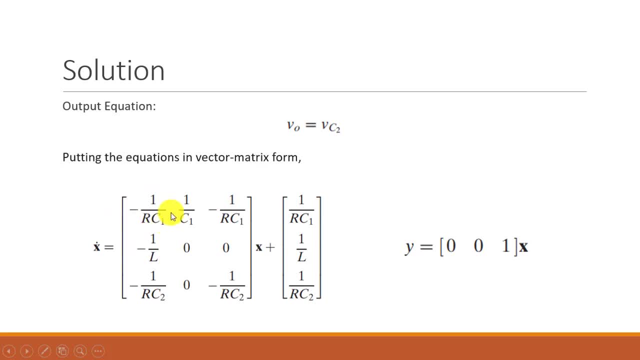 the very first equation has minus 1 over RC1 as the coefficient of VC1, which is which would be the part of X matrix, and this would be filled from the values of VI that were being added as the constants. So you can see that VI has 1 over RC1 coefficient in the DVC1 by DT equation. 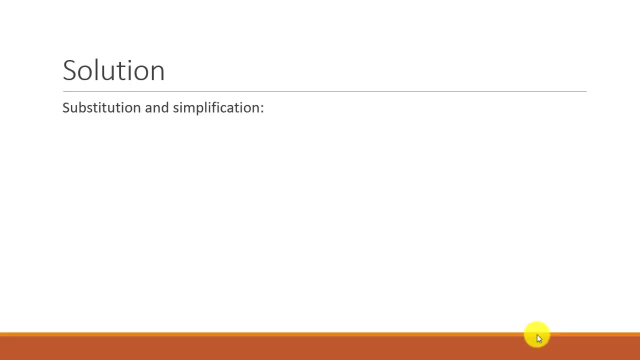 and you can see, I'm sorry, and you can see that, yes, my 1 over RC1 is the value that is being multiplied with the U, which is the input VI. So, in the same trend you will follow, you will fill all these matrices: matrix A, matrix B and 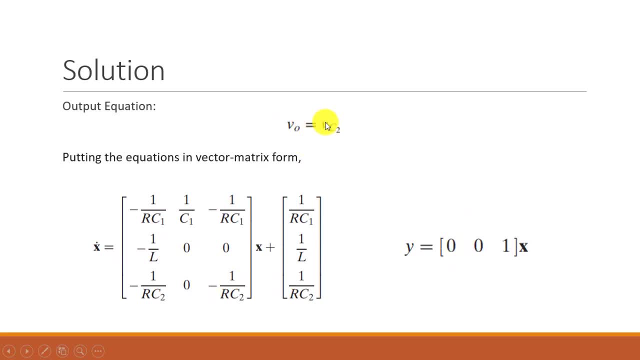 the matrix C would be filled using this information, which is the output equation. So in this way you will find out the state-space representation of any electrical network. you first of all need to find out the state-space variables, and then you need to find out the exact equations that you